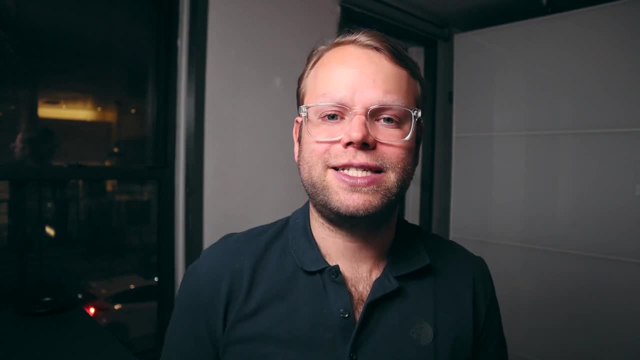 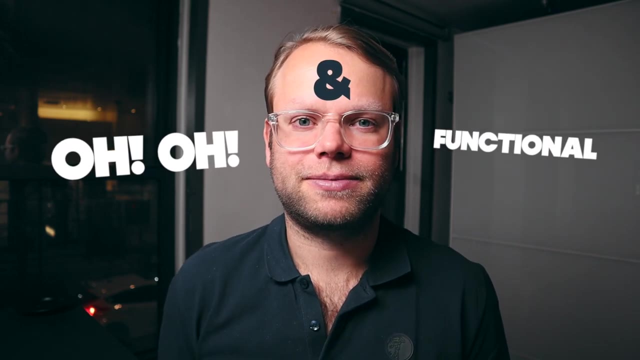 And I think that would probably have made Scala's adoption easier sort of in the long haul, because a lot of people get confused by being able to do both OO and functional. Yeah, we'll do that. 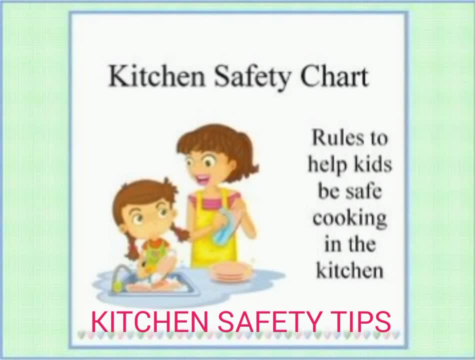 Hello children, today we have brought a new video for you and that talks about some kitchen safety tips. Hope this would be helpful for you, especially when you are in kitchen. So let's see what are the safety rules or what are the safety tips when you have to follow in the kitchen. 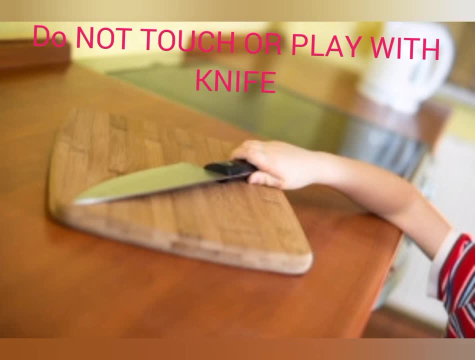 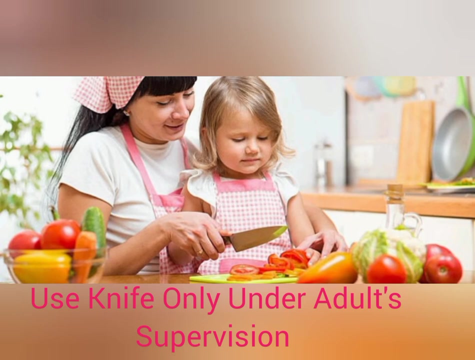 Do not touch or play with knife. You must not touch the knife, you must not play with the knife and you must also not touch any sharp object. Right Okay, if you want to know or learn how to cut vegetables and fruits, you should use the knife only under adult's supervision. 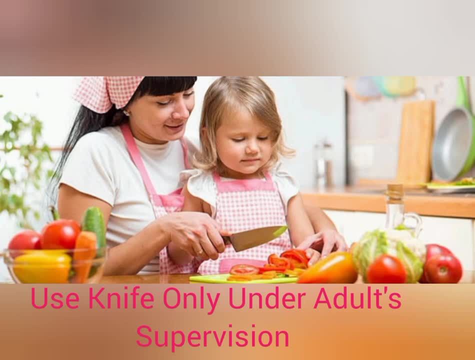 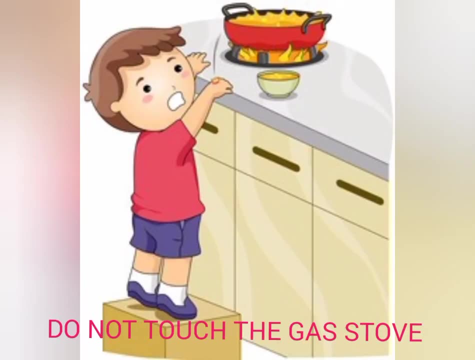 It means your parents must be there when you are trying to use the knife. Do not touch the gas stove. Okay, look, you should never touch the gas stove, Especially when it's on or when something is being cooked. Then what else? 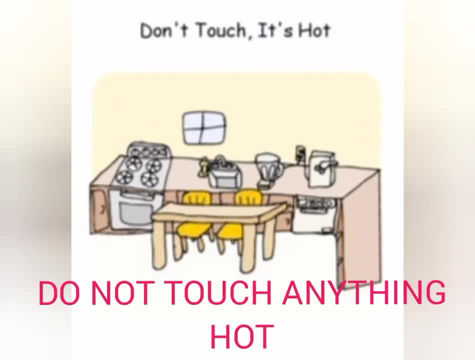 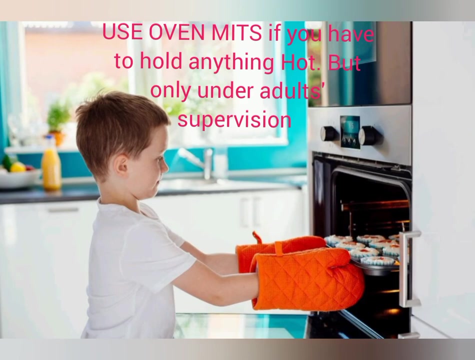 Do not touch anything that is hot. Okay, there are many objects, many things which are hot and your mother or father might have cooked recently and which is still hot. You should not touch them If you have to. if you have to touch anything that is hot, always use oven mitts. 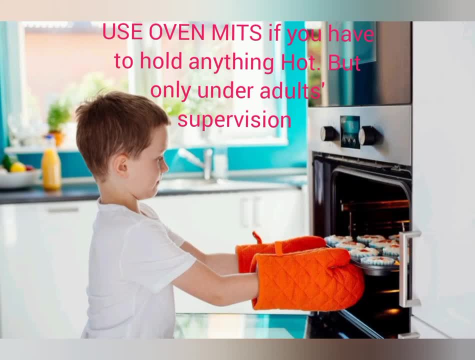 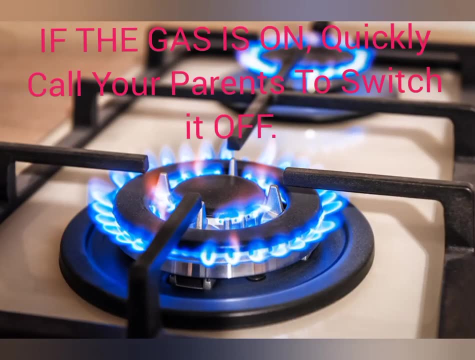 Okay, Which are very safe to hold the hot object, but also only under during when your parents are present. If the gas is on, quickly call your parents to switch it off. Make sure you do not switch the gas off or do not switch it on by yourself.